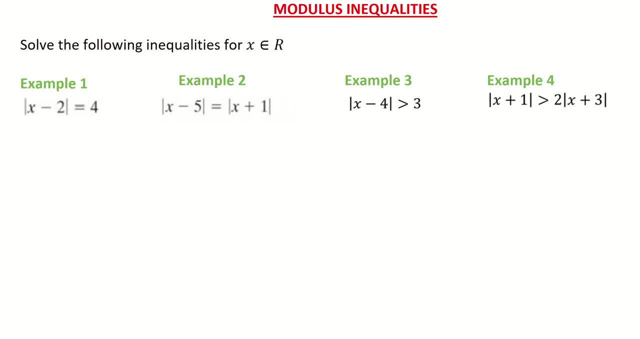 In this video we're looking at modulus inequalities. We're going to look at four examples. The first two are using an equal sign, so they're a little bit easy in nature and then they get a little bit harder in example three and four. Just a little bit of revision of what 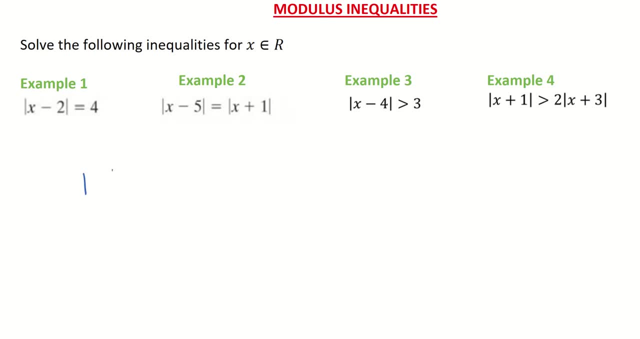 modulus is. So these parallel lines are standing for a modulus. so if i'm looking for the modulus of, say, five, it basically turns your value into its absolute value, so it's positive value. so the modulus of five is five. Now that could have also been the case the modulus of negative five. 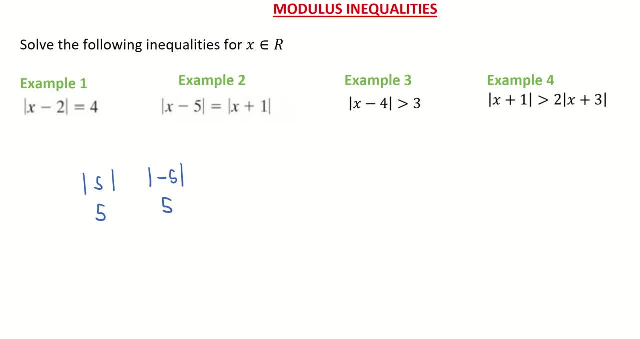 which basically means you turn your value into a positive value, so five. so it's usually got to do with, maybe, areas of triangles. you might have seen the modulus or the values for lengths of coordinate geometry. So that's what the modulus is doing for us. so if we had another example, 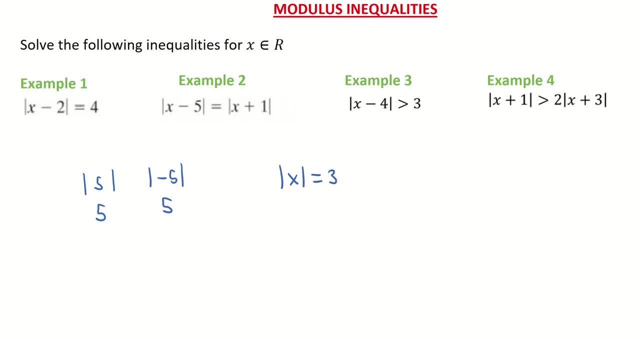 here the modulus of x is equal to 3. technically, the values for x there are negative 3 because the modulus of that is 3, but I could also use x as positive 3, because the modulus of positive 3 obviously has to be 3.. So there's two values there for x. Now the easiest: 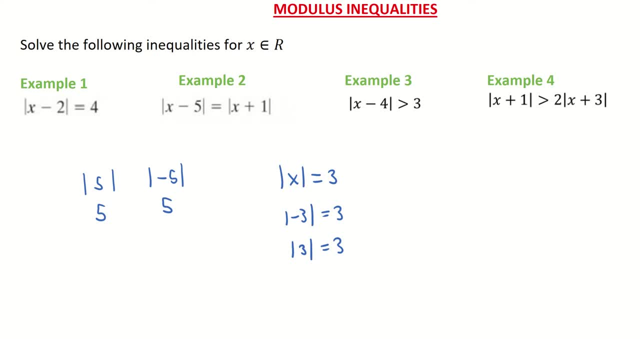 way to find the values for x here would be to square both sides. So what I mean by that is, if we keep our basic example here of the modulus, of x is equal to 3.. So in order to find those two values of x, the easiest way is to just come along and square both sides. because when we square the x, 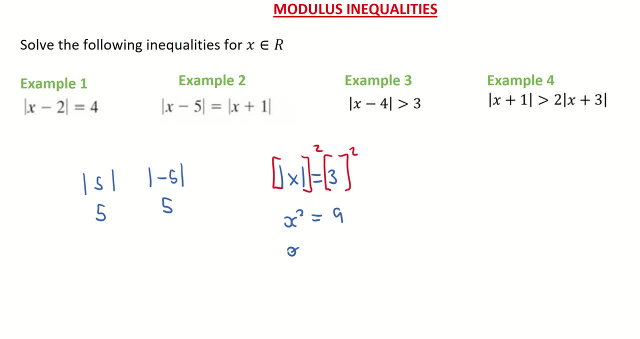 we get x squared and we square the 3 and we get 9, and the square root of 9 is plus or minus 3.. So that's how we're going to solve these 1,, 2,, 3, 4 examples of modulus: We're going to square. 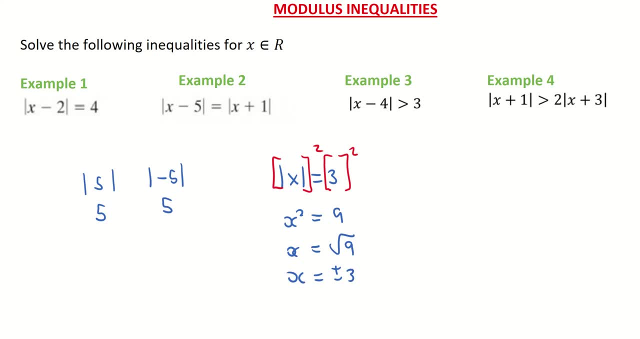 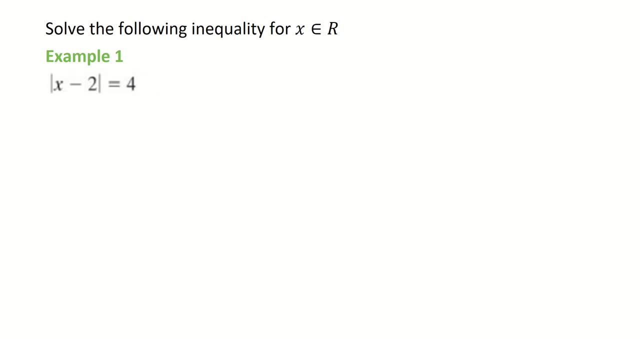 both sides and solve for x basically. So let's have a look now at example 1.. So it's asking us to solve the inequality for x, an element of the real number, So real numbers are positive. So we're going to solve for x, an element of the real number, So real numbers are. 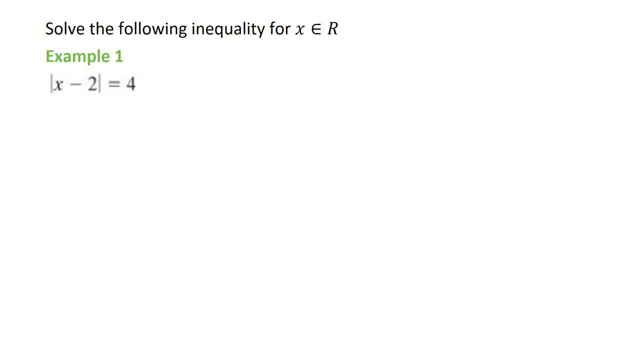 positive and negative, whole, or rational numbers, so fractions and decimals. So the method of doing this is to square both sides. So I'm going to go: x minus 2, all to be squared is equal to 4 to be squared. Multiplying x minus 2 by itself is my next step, because a square means you multiply it. 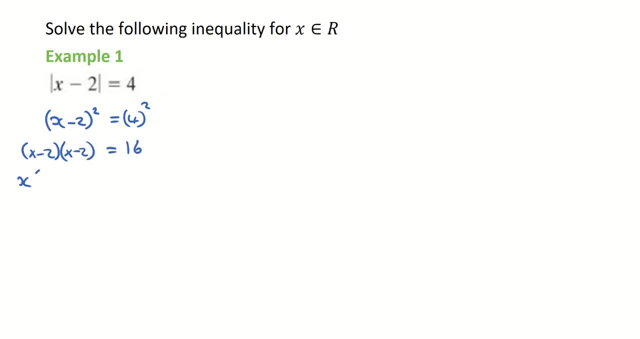 by itself and 4 squared there will give you 16.. So first term by my second bracket and second term by my second bracket is equal to 16.. I'm multiplying in my brackets then. So first term by second term and so on is going to give me x squared minus 2x minus 2x and negative. 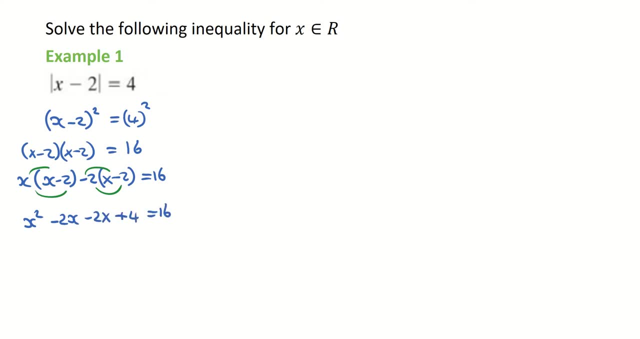 2 by negative 2 will give me a plus 4 is equal to 16.. If I move that 16 over or subtract 16 from both sides, I'm getting x squared minus 4x plus 4 minus 16 is equal to 0.. So my quadratic is x. 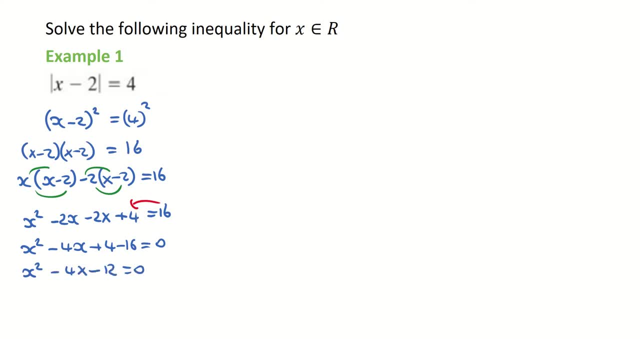 squared minus 4x minus 12 is equal to 0.. So I'm trying to find the values of x. so I need to solve my quadratic here So you can use your guide number, trial and error, using your two brackets or your minus b formula, your quadratic. 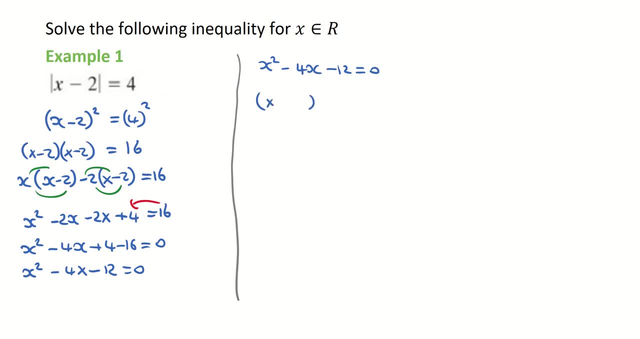 formula. I'm going to just do the two brackets here. I think it should be straightforward enough. So it's equal to 0.. So the multiples of minus 12 to get to minus 4 are going to be minus 6 and a plus 2.. So they're my factors and when I solve those I get x is equal to 0. 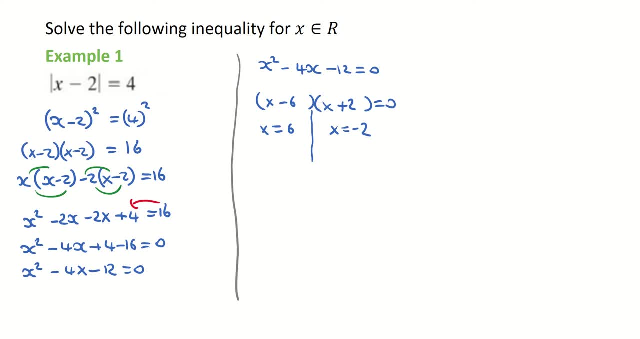 x is equal to 6 and x is equal to minus 2.. So therefore, my two values for x are positive 6 and negative 2. And you can always check these by subbing them back in to your modulus. So that's example 1.. Let's have a look there at example 2.. 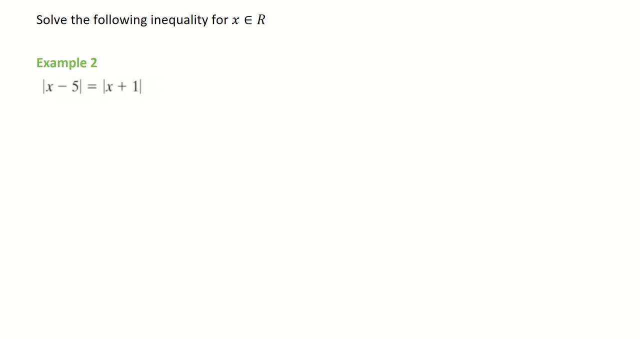 So solve the following: inequality for x an element of r, x minus 5 modulus is equal to modulus of x plus 1.. So the process once again is to square both sides. So it's x minus 5 to be squared is equal to x plus 1 to be squared. Squaring something means you multiply it by. 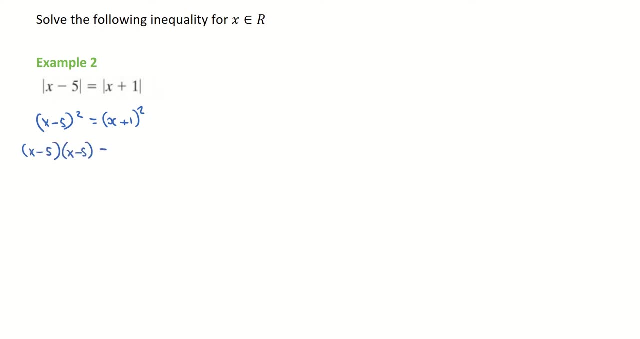 itself. So x minus 5 multiplied by x minus 5 is equal to x plus 1 times x plus 1.. So multiplying out your bracket, So first term by the second bracket and second term by the second bracket on both sides of the equal. So it's a little bit algebra heavy here really, So just take your time. 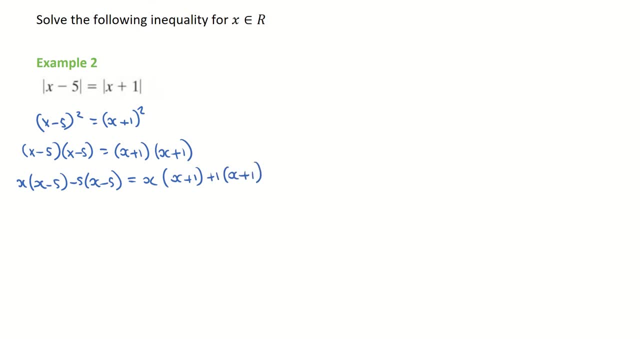 as you multiply out your brackets. So, multiplying out the first two, you get x squared Minus 5x minus 5x minus 5 by minus 5 is a positive 25.. And on the right hand side of the equals we get 1x plus 1x plus 1 by 1, which is 1.. Tidying it up a little bit: x squared minus 10x. 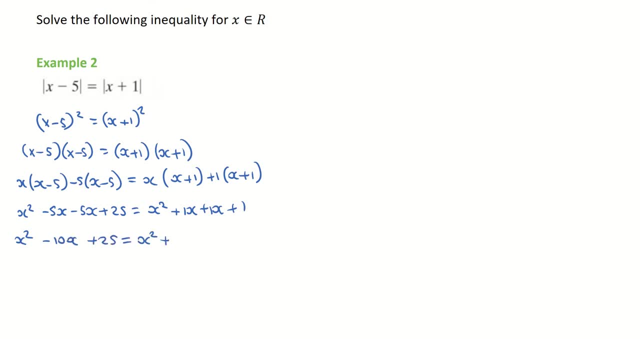 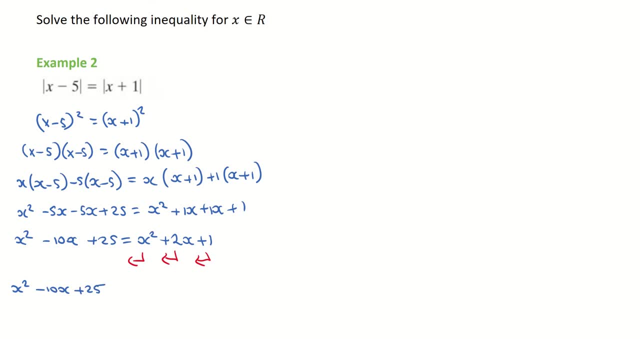 squared minus 10x plus 25, and then I'm moving over the x squared to become a negative x squared, negative 2x plus 1 will change to a negative 1. And that is now going to equal to 0 on the right. 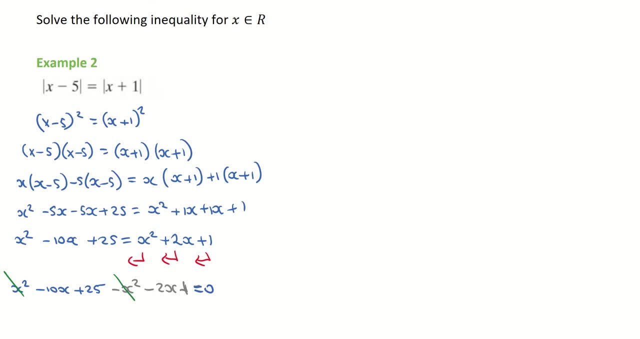 hand side. Hopefully you can spot here that the x squared minus x squared will cancel out. So that's leaving me with minus 10x. minus 2x is minus 12x plus 25x, minus 5x, minus 5x, minus 5x. 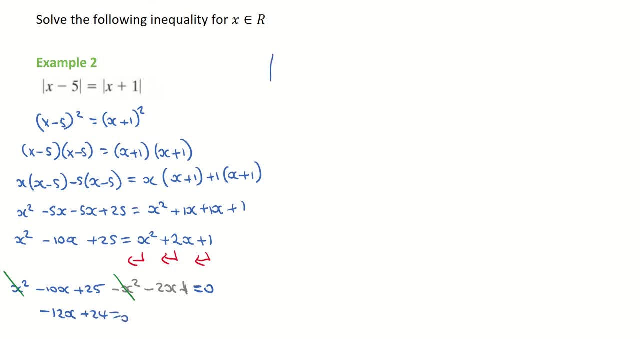 minus 1 is plus 24 is equal to 0.. I need to solve that linear equation now, So let me just rewrite it up here. So I'm going to have x's on one side and numbers on the other. So subtract 24 from both sides will leave me with minus. 12x is equal to negative 24, and dividing across by 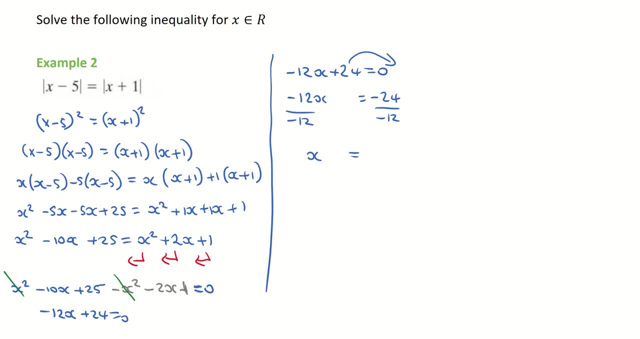 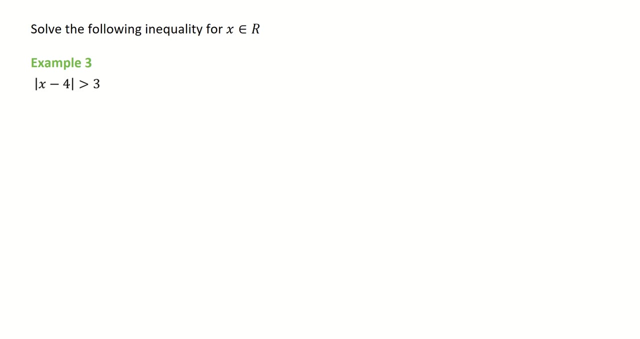 negative 12 will give me a value of x as positive 2. So there's only one value for x on example 2. And that's x is equal to 2.. Looking at example 3, next Solved following: inequality for x, an element. 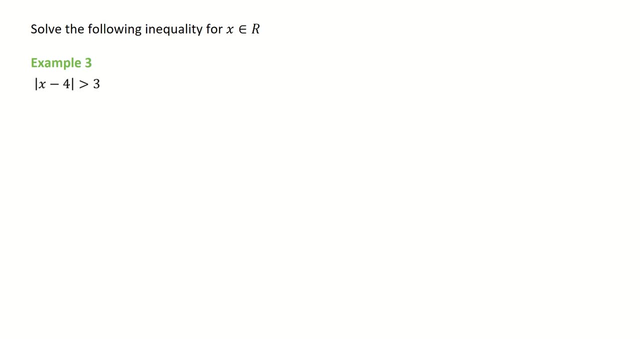 of or. So it's now getting into a greater than symbol rather than the equals, but we carry these out in the same fashion. We square both sides, So it's x minus 4 all to be squared. greater than 3 to be squared. Squaring something once again means you multiply it by itself. So x minus 4 by x minus. 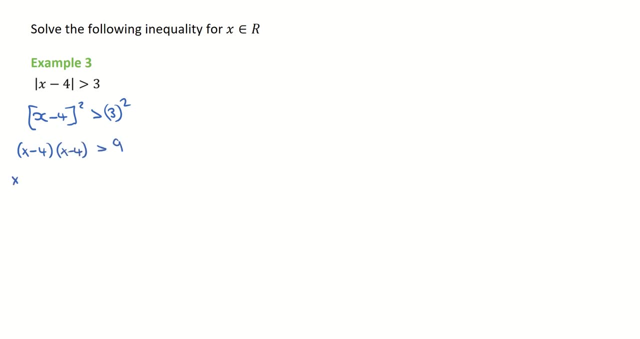 4 is greater than 2.. So it's x minus 4 by x minus 4 is greater than 2.. So it's x minus 4 by x minus 3, which is 9.. So, first term by my second bracket, second term by my second bracket, greater than 9. 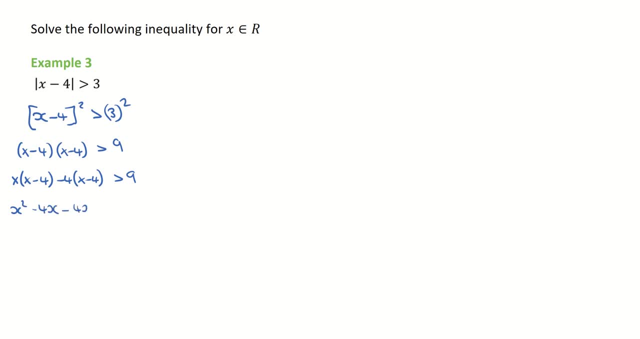 which is giving me x squared minus 4x. minus 4x plus 16 is greater than 9.. So just tidying up this now a little bit, is giving me minus 8x plus 16.. And if I subtract the 9 from both sides or move, 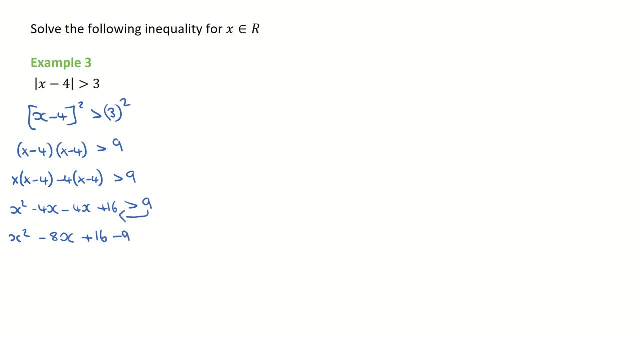 over that 9, that's leaving me with a negative 9 greater than 0, because we can only solve our quadratic equation. So if I subtract the 9 from both sides or move over that 9, that's leaving me equations when it is greater than or less than, or equal to 0. So that's my quadratic equation. Now, 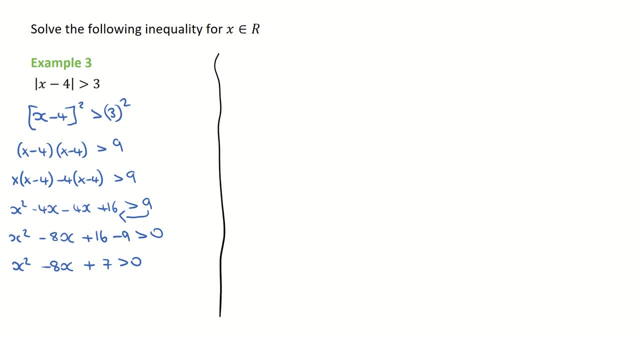 I'm going to come up and solve my quadratic. So again, guide number minus b, formula, two brackets, whichever way you want. So what we're trying to do first of all now is find the roots of the equation. So I'm going to let it equal to 0 here, just to solve the roots, because I'm looking for. 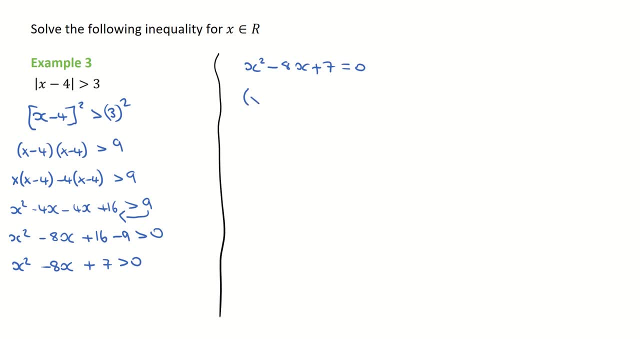 where it crosses the x-axis, So when that's equal to 0.. So my two brackets, x and x, and equal to 0, and the multiples of 7 are 7 and 1 and a minus and a minus, because minus by minus gives me plus. So the roots are x is equal to 7 and x is equal to. 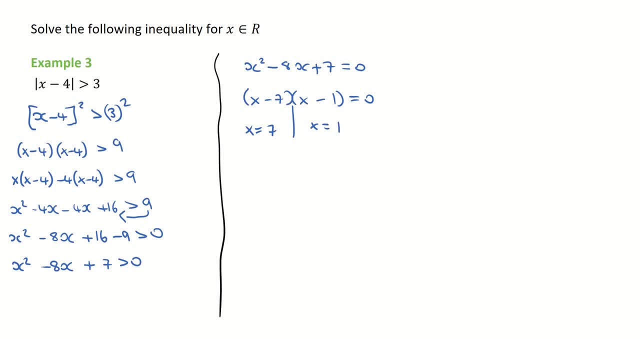 positive 1.. So what does that mean? So if we come back, if we come down here, just do a little sketch of this and it's crossing the x-axis at number 1 and number 7 and it's a positive quadratic. So maybe look something like that. So we're looking for where it's greater than 0.. So, greater than 0. 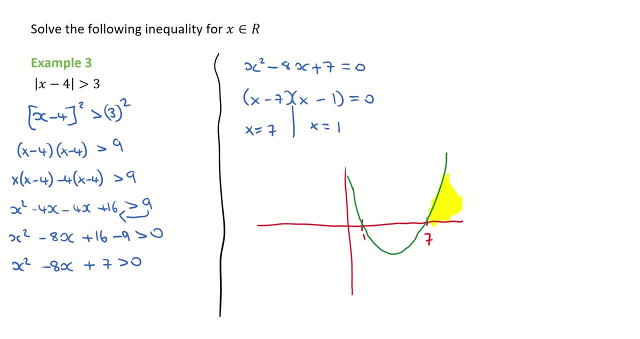 is above the x-axis. So it's this portion of my graph here and this portion of my graph here. So the values for x here are going to be x greater than 7.. So I could use 7, 8, 9, 10, 11, all the way to. 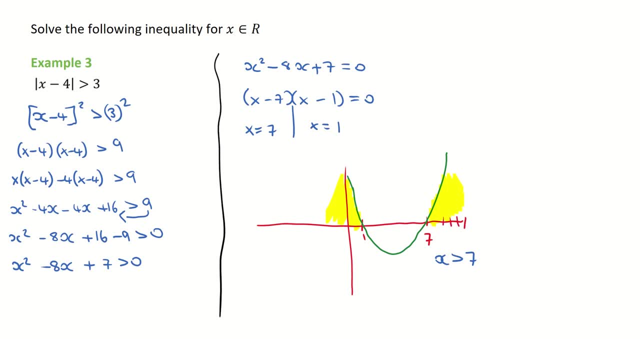 infinity, So anything basically in this yellow portion here. But I could also go down to anything below 1. So x less than 1. Because I can do that, So I could do that, So I could do that, So I could. 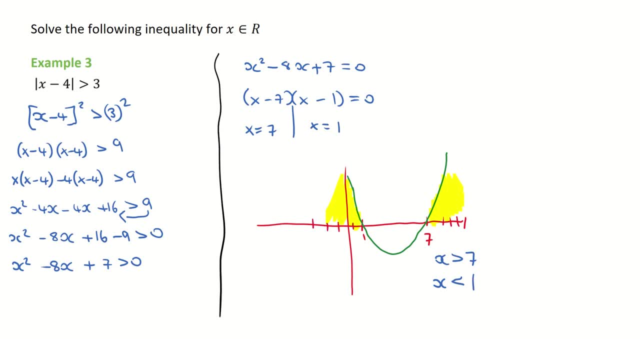 include 0 minus 1 minus 2 minus 3.. All these values here The only values I can't use- are anything between 1 and 7.. So that's example 3 done. Let's have a look now at example 4.. 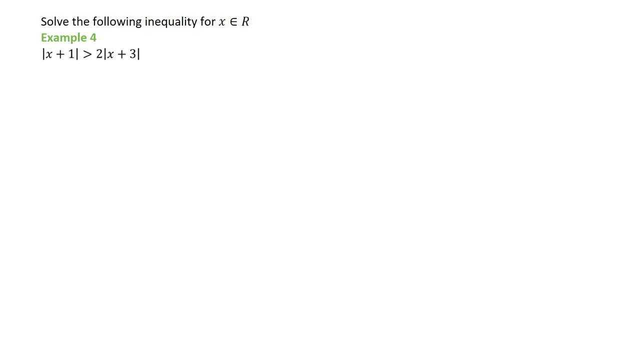 Solved following inequality for x, an element of the real numbers. So again we have an inequality here, modulus on both sides, So we need to square both sides to deal with the positive and negative of that inequality. So that's going to give me x. 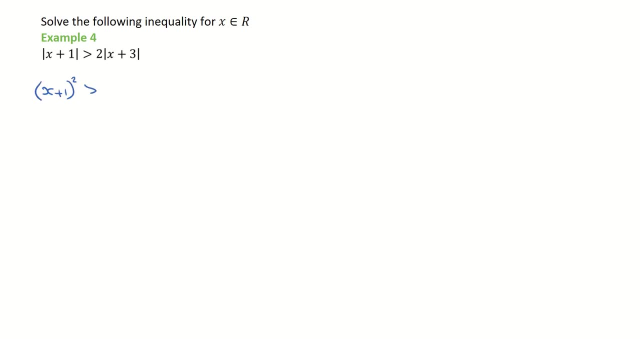 x plus 1 on the left hand side And I'm going to square that And that's going to be greater than 2 times x plus 3, all to be squared. So what you're doing here is you'll have to square the 2 and 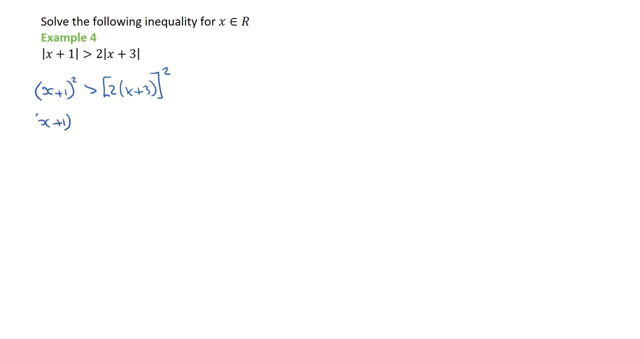 then you'll have to square the bracket. So we can write that out, if it makes it easier. So it's x plus 1 to be squared, greater than 2 to be squared, and the x plus 3 to be squared. So I'm going to do. 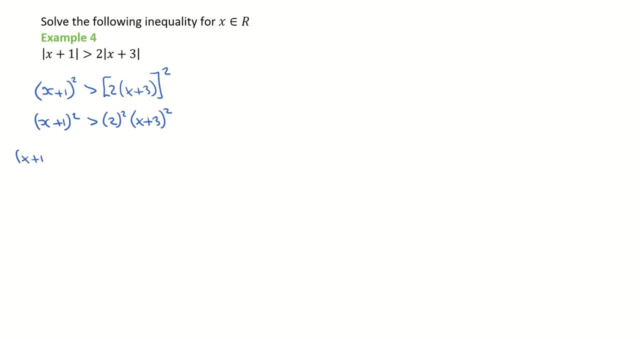 them separately. So on the left hand side that'll give me x plus 1 times x plus 1.. And on the right hand side 2 2's, And then I need to multiply out my 2 brackets. So I'm just going to use square brackets here, just to keep them. 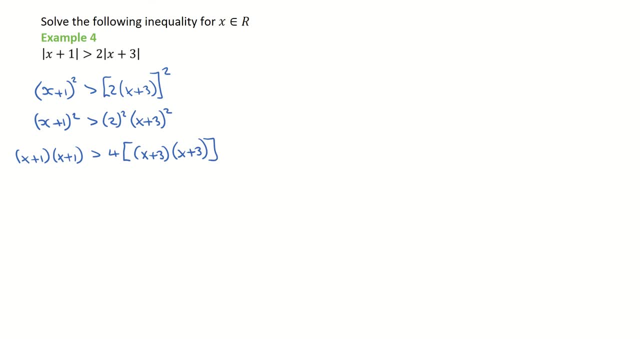 separately And I need to times them by each other as well. So first term by my second bracket, and then second term by my second bracket, greater than 4 times the x times the second bracket, and then the plus 3 by the x plus 3.. So just take your time with your multiplication here. Now I'm just going to. 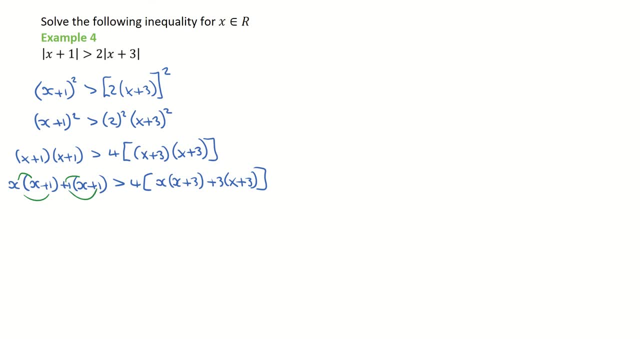 multiply in my bracket here, So use the arrows if it helps. So that's going to give me x times x plus 3.. So that's going to give me x by x is x squared plus 1. x plus 1. x plus 1 greater than 4 times x by x is x. 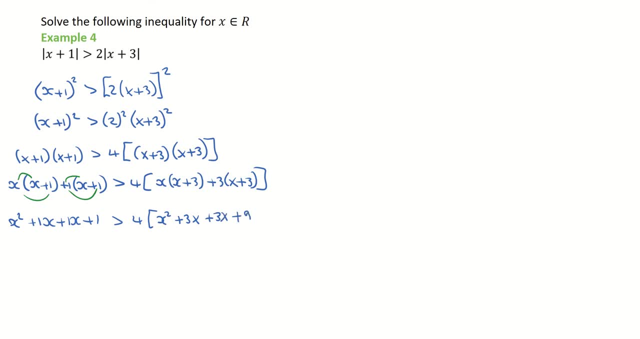 squared 3 x, 3 by x is 3 x and 3 by 3 is 9.. Just timesing in that 4 now into this bracket, multiplying it in, is going to give me greater than or equal to 4 x squared. Well, that 3 plus 3 is 6 and 6 by 4 is 24 x and 4: 9's is 36.. 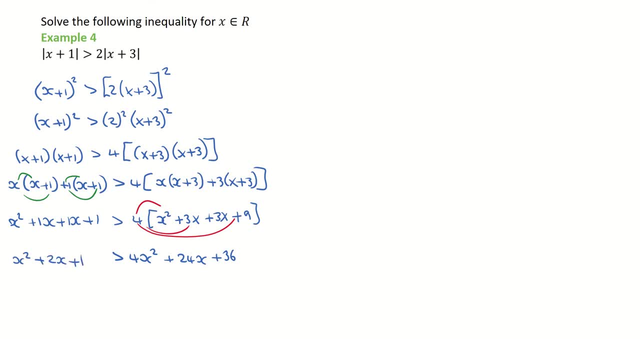 And on the left I have my x squared plus 2, x plus 1.. Tidying that up, now I'm going to move everything to the left hand side, So minus all of this quadratic, in other words. So that's going to give me x squared plus 2 x plus 1.. 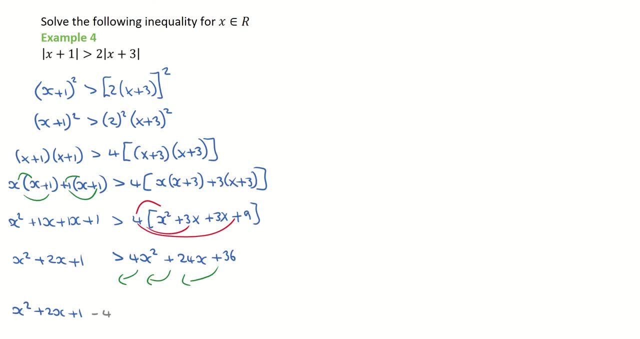 And as I move them over, let me just change the colors here, So that'll be minus 4 x squared, minus 24 x minus 36.. And that will all be greater than 0.. So Grouping terms I have: x squared. minus 4 x squared will give me a negative 3 x squared. 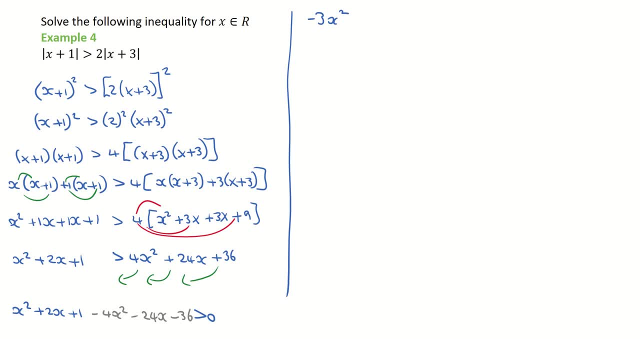 I have a 2 x minus 24 is a minus 22 x. and then I have my 1 minus 35, which are 36, is minus 35, greater than or equal to 0.. So make it a little bit easier, I'm going to multiply across by negative 1 to change the signs. 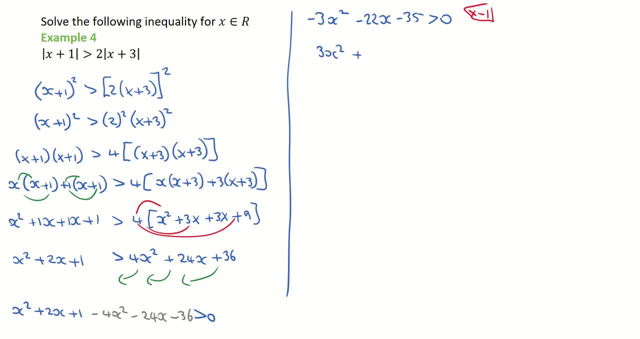 So that's going to give me positive 3 x squared positive 23.. 2 x and a positive 35.. But remember, when you multiply across or divide by a minus, you have to change the direction of your inequality sign. So my inequality sign there is flipping. 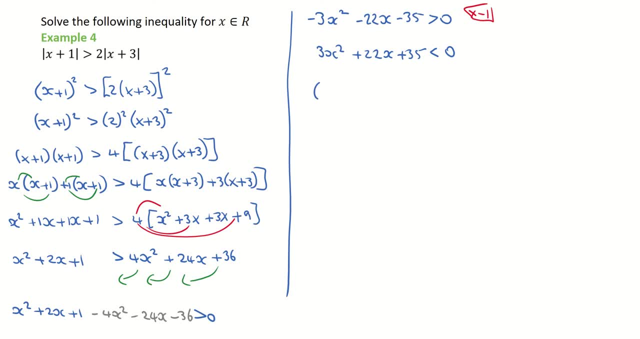 So now I'm looking to factorize this, So using your minus B formula, if it's a little bit easier, or you can use your, your two brackets. either way, Let's see what we get. So the factors of 35 that are multiplying: 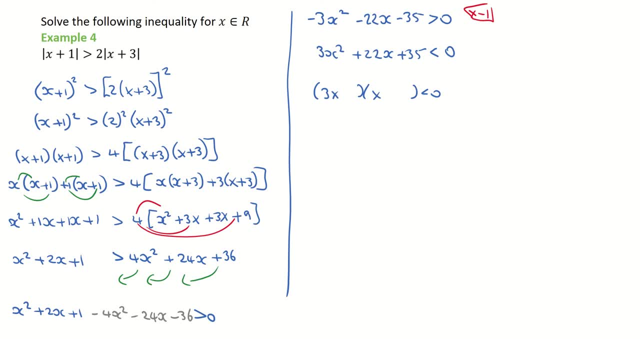 Multiplying to 35 and adding to 22.. We could have a 5 and a 7 and positive and positive. so that would give me 15 plus 7 is 22.. Yeah, So they are my solutions, So they're my factors solving these. now I get 3: x is equal to minus 7, x is equal to minus 7 over 3, or 2 and 1. third, 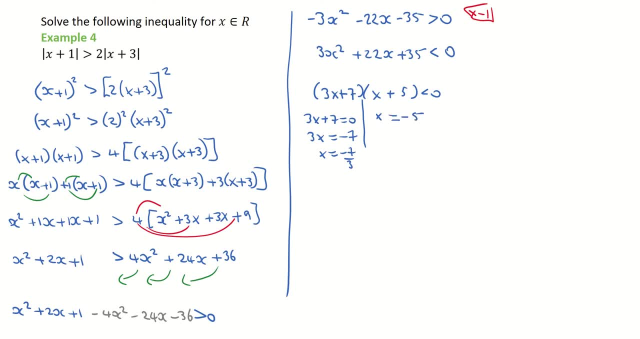 And my second root is going to be x is equal to negative 5.. So they're my roots where it crosses the axis. So technically there, when I'm solving that, I'm going to have that equal to a 0.. So let's see the question again. wants us to solve the inequality. 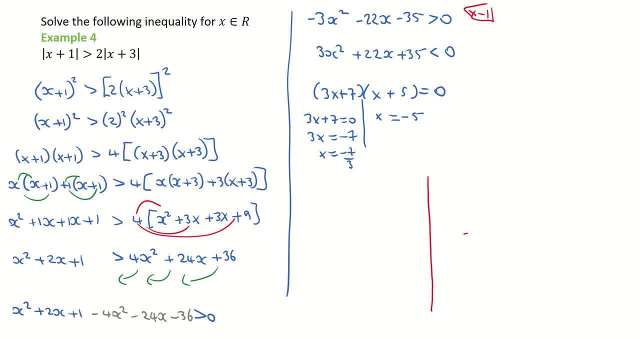 So there's a range of values here, So I'm just going to sketch this out once again and see how it looks. So minus 5 would be down here, minus 2 and a third probably around here. So minus 7 over 3 and it's a positive quadratic.